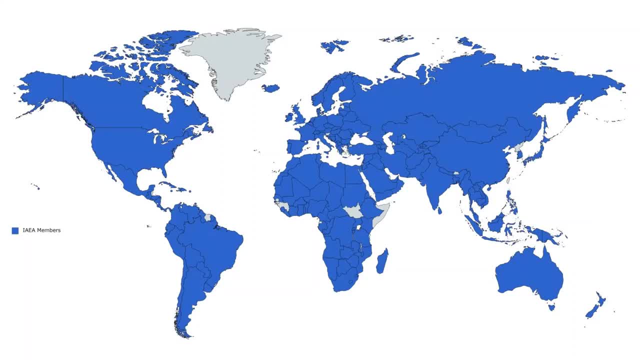 And, like the Non-Proliferation Treaty, membership in the IAEA is very widespread. Almost this entire map is blue And that's because there are a lot of benefits to being a member of the IAEA and very few downsides As a consequence. the exceptions on this map: 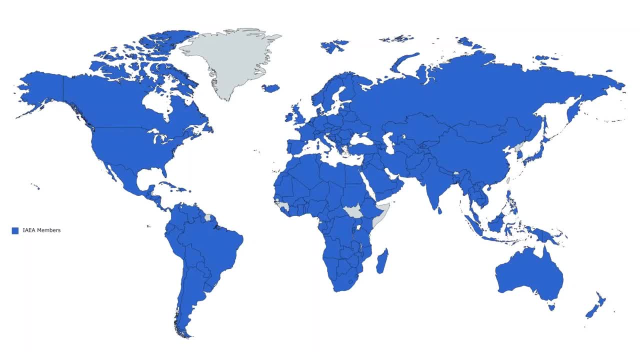 are few and far between. One of those exceptions is North Korea, although actually North Korea was once a member of the IAEA. But it's not the only exception. The IAEA is also a member of the IAEA. You'll recall that in 1994 there was a falling out. 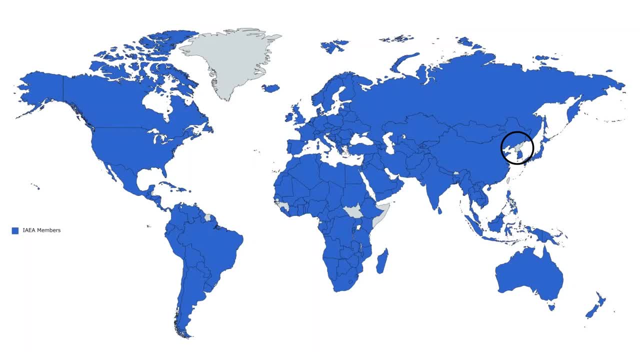 between the non-proliferation regime and North Korea. when it was alleged that North Korea was violating some of its safeguard agreements, North Korea pulled out of the IAEA in response and has never returned. Another entity not in the IAEA is Taiwan, Although, like North Korea, 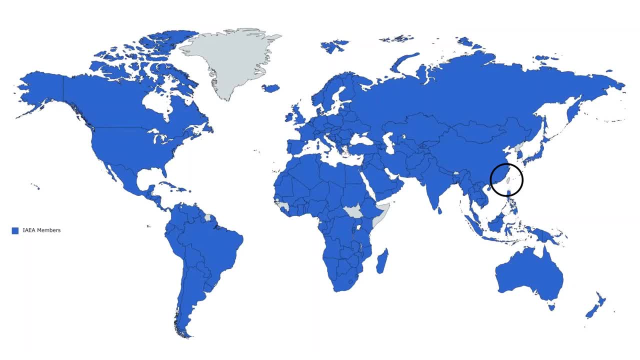 Taiwan was once a member. However, when China's representation in the United Nations transitioned away from Taiwan and to mainland China, Taiwan had to leave the IAEA And, like North Korea, it has never returned. A few notable countries that are in the IAEA are India, Pakistan and Israel. 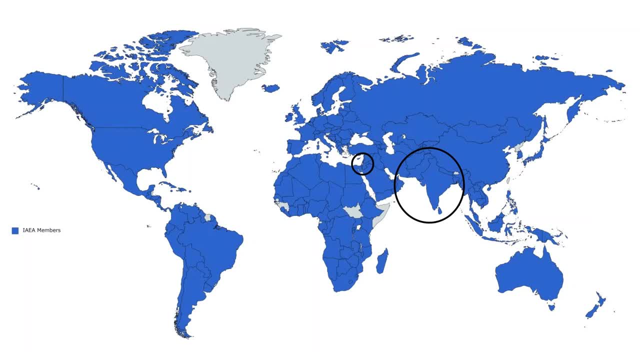 That might be somewhat surprising, given that those countries are not a member of the Non-Proliferation Treaty as a consequence of them having nuclear weapons. However, the most important issue is that the IAEA is not a member of the IAEA, But the IAEA predates the Non-Proliferation Treaty by 13 years And, perhaps surprisingly. 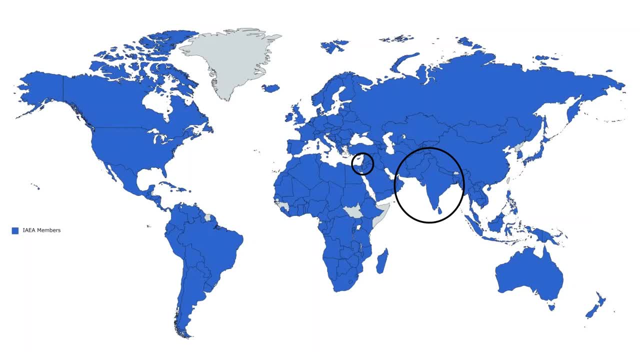 compliance with the Non-Proliferation Treaty is not a requirement for membership in the IAEA. As a consequence, these countries can still be members despite their status with the Non-Proliferation Treaty. As a result, the only other countries that are not members 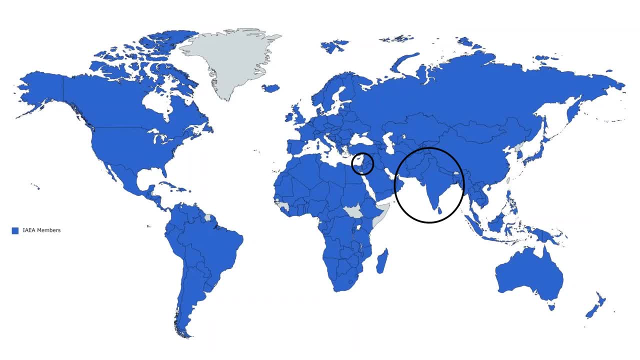 tend to be very, very poor. The structure of the IAEA is very similar to that of the United Nations, though the IAEA itself, perhaps surprisingly, is not a subsidiary of the UN. They do, however, often work together, given that they have common goals. 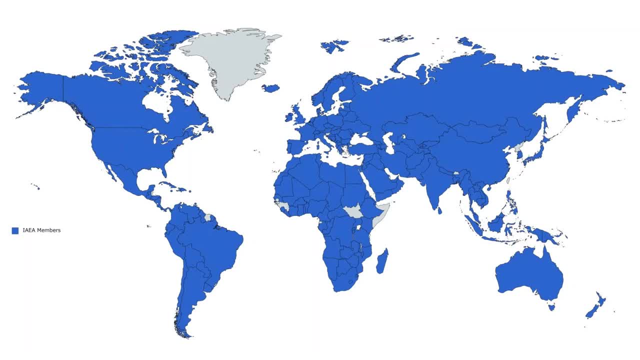 The main body of the IAEA consists of every member state. This is roughly equivalent to the United Nations General Assembly, But like the United Nations, there is a body within the IAEA that serves as a governing board. Membership here is much more exclusive. 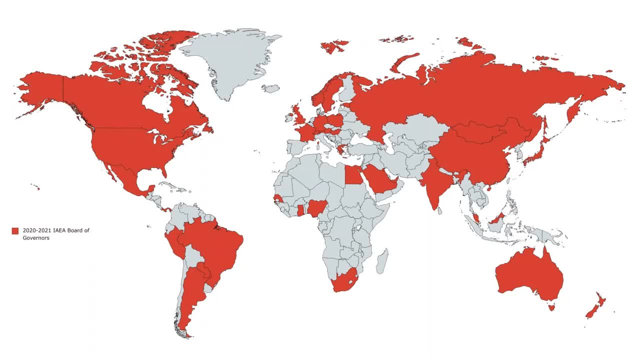 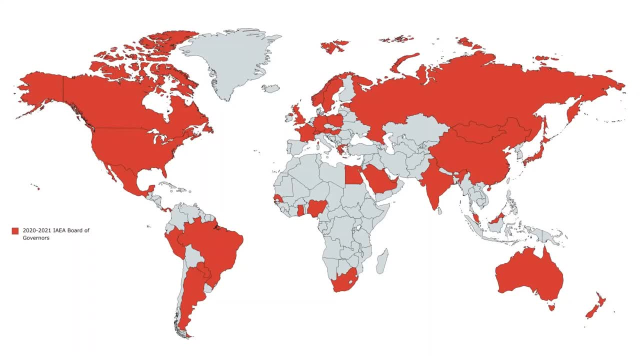 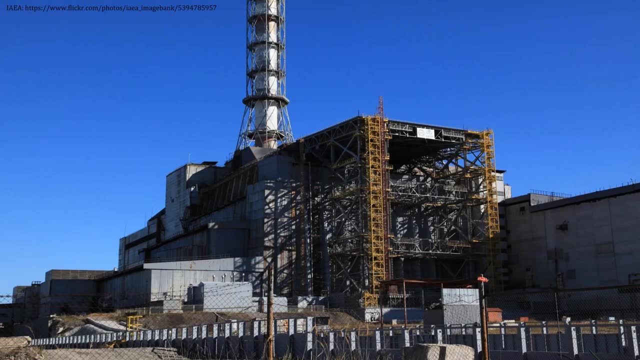 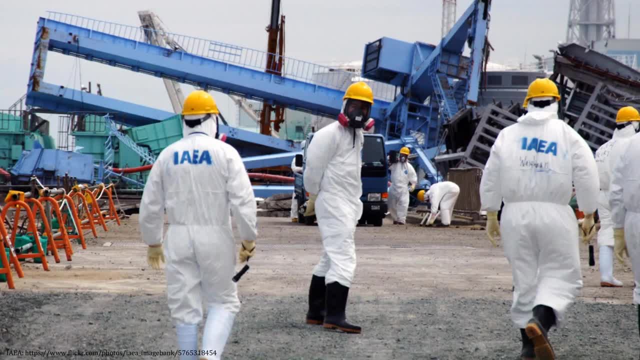 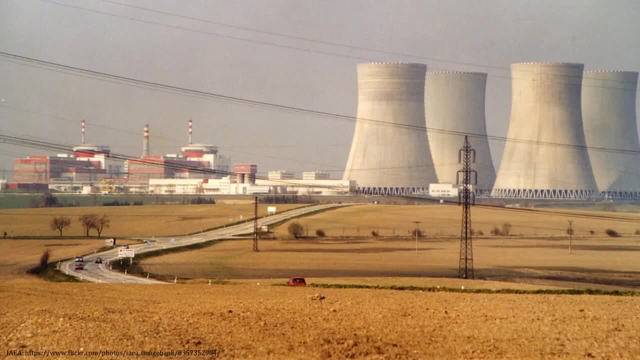 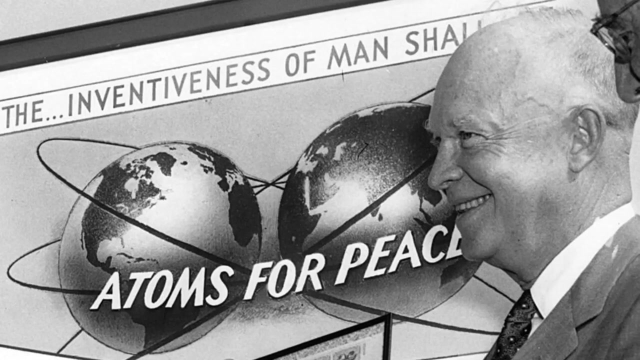 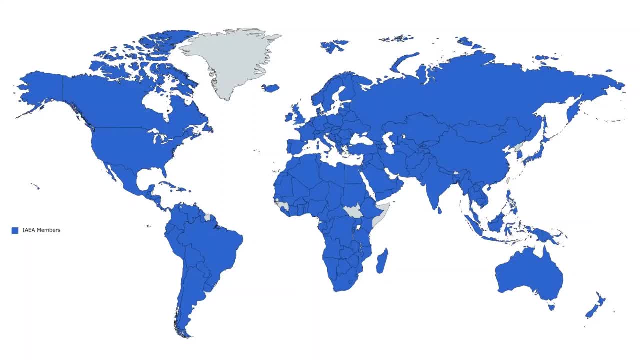 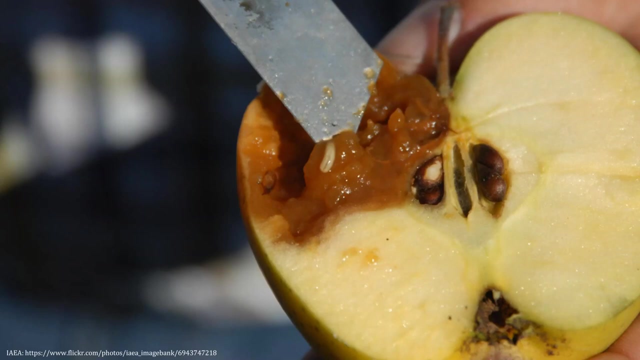 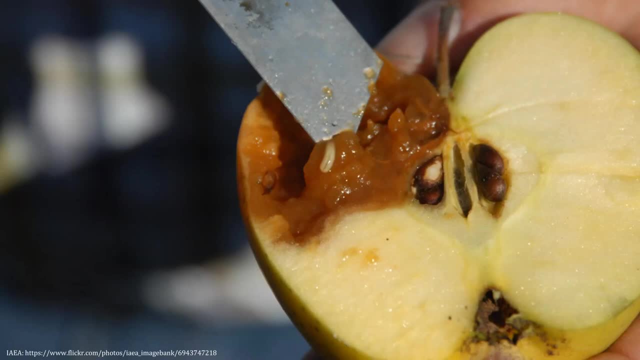 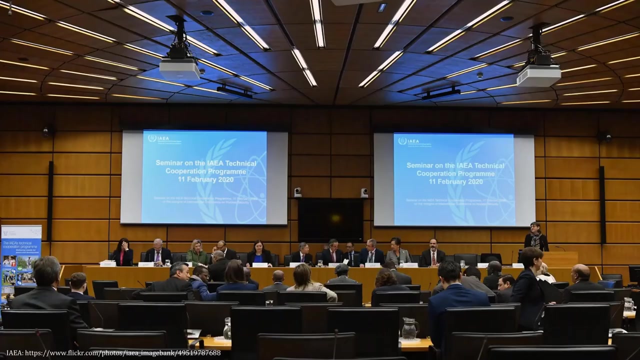 essentially render them infertile and then reintroduce them to their natural habitats to try to mate and crowd out the fertile versions of those species. This results in overall lower pest quantities, which can increase crop yields. These types of projects get funded under the IAEA technical program. 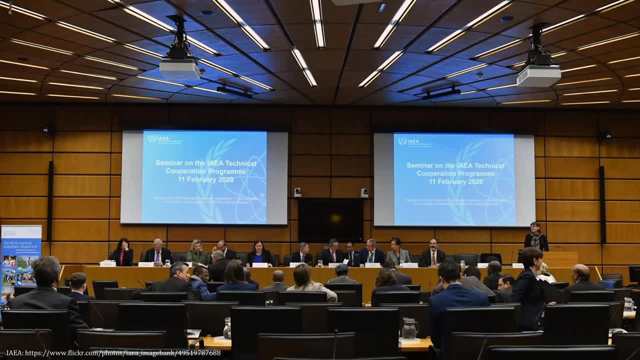 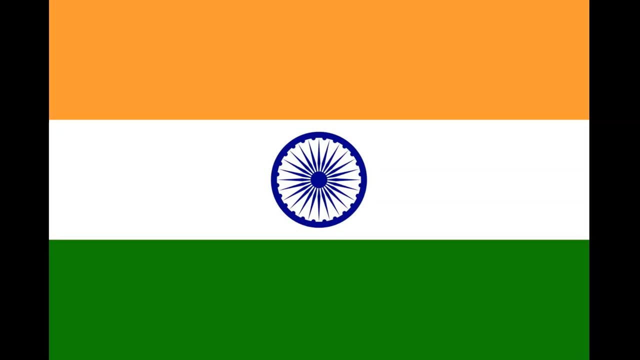 However, getting help today is very different from how countries might receive help in the past. The big day of reckoning came in 1974, when India did its Smiling Buddha test- Much of the infrastructure that India used to create that nuclear weapon. 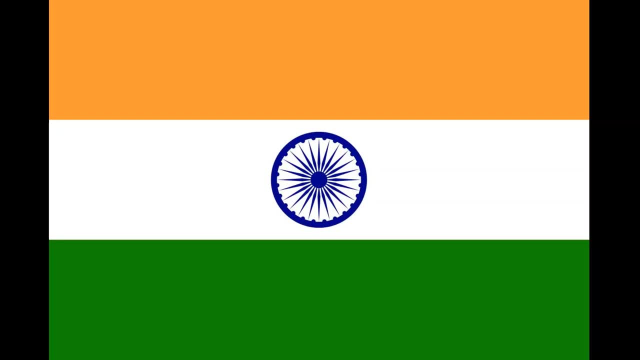 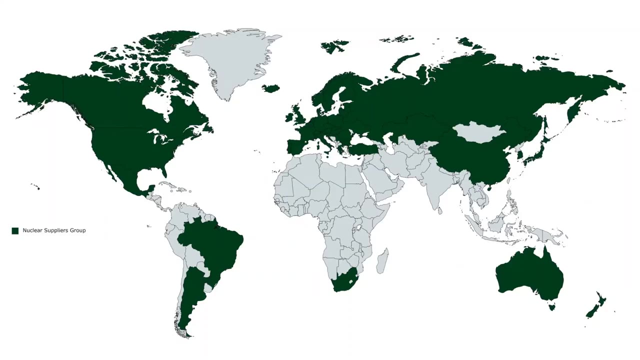 was through Atoms for Peace-style programs And as a result, the international community had to rethink how these programs were run. Two big initiatives came out of that. The first is the Nuclear Suppliers Group. The Nuclear Suppliers Group is a group of people who work in the nuclear industry. 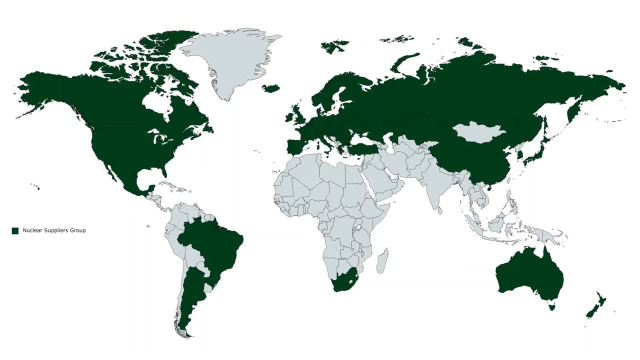 This is a committee of countries that have the technical capacity to help others with nuclear technology. By forming this committee, they hoped to create regulations to make sure that technologies that were shared would not make it cheaper and easier for other countries to develop nuclear weapons. 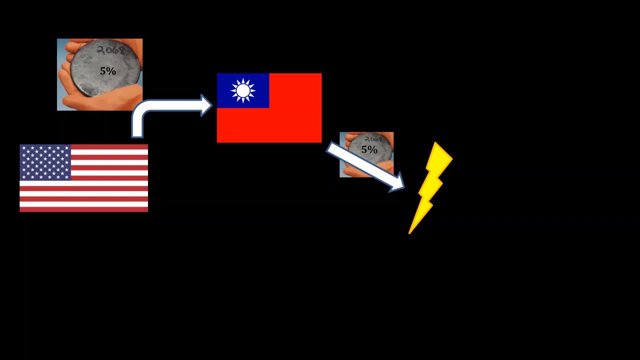 The second thing that the regime has done is become more careful with what materials are handed out. Imagine you're a recipient like Taiwan And you need to have fuel to run your nuclear power plants. The way this works today is as follows: The United States will give you 5% enriched uranium fuel. 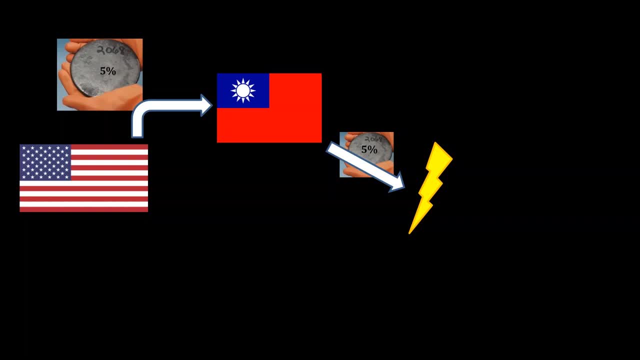 that contains 5% of the fissile uranium-235 atom to the recipient. The recipient will then put that into their nuclear power plant and create energy. Running the power plant creates nuclear waste. The recipient country is then the nuclear power plant, And the recipient country is then supposed to take that nuclear waste and ship it back to the donor country. 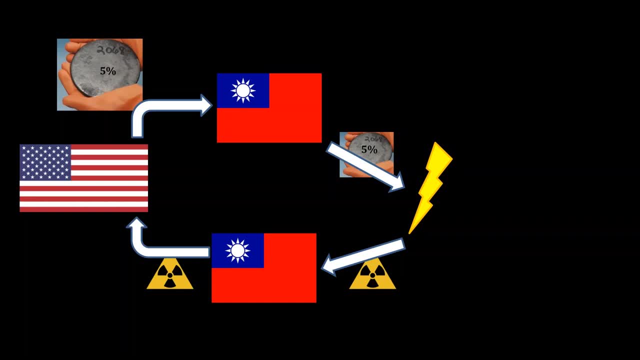 The donor country can look into that waste material and verify that everything that is supposed to be there is actually there And what has been handed back is consistent with the recipient country having run the nuclear power plant for energy. If all of those boxes are checked, then the cycle begins anew. 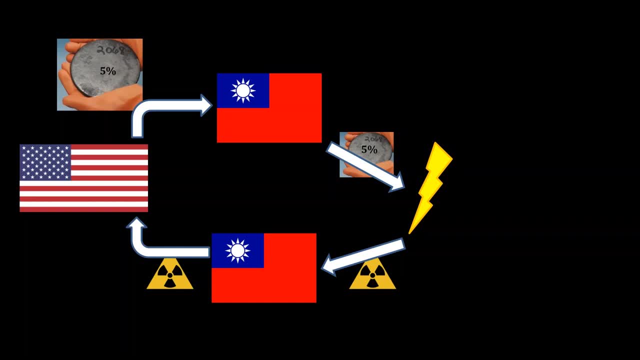 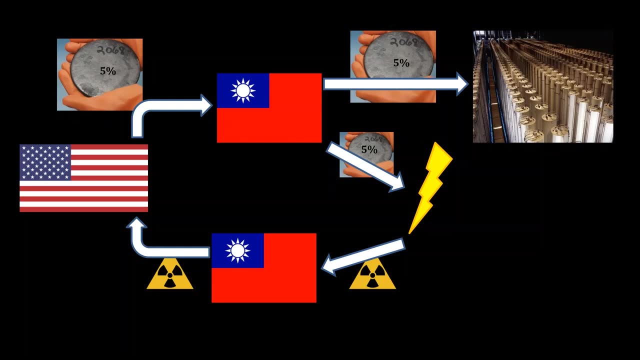 with the donor country giving a new round of fuel to the recipient country. There are only two ways to do this. There are only two weak links here, And even then they're not all that bad. One issue is that the recipient could take the fuel and not run it through a power plant. 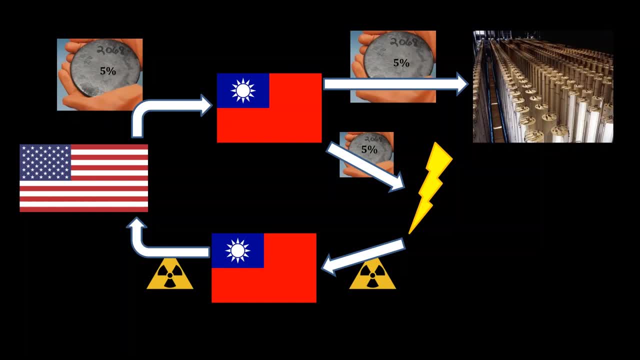 Could instead try to use that to help build a bomb. The problem is that 5% enriched fuel really isn't good enough. This is just low enriched uranium, And you need highly enriched uranium, containing about 90% uranium-235, to actually build a nuclear power plant. And that's not even a nuclear weapon. So even if you had this fuel, you would still need a uranium enrichment facility to get up to the point of having a fissile bomb. To be fair, having 5% enriched uranium is better than having unenriched uranium. And indeed it is more difficult to get from naturally occurring uranium to 5% uranium than it is to go from 5% to 90% enrichment. Nevertheless, having 5% enriched uranium does absolutely nothing for you if you want to build a nuclear weapon. 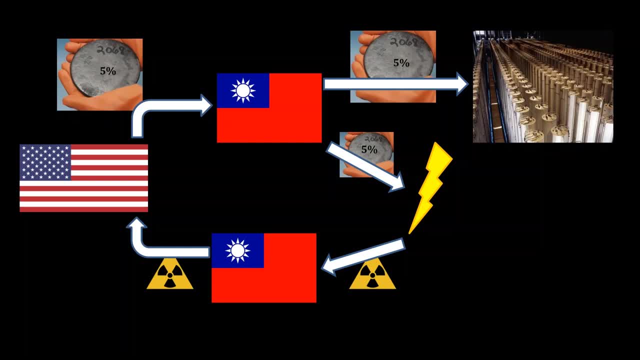 if you don't have these uranium enrichment facilities. This stands in contrast to how previous agreements worked, where some nuclear power plants would actually operate on highly enriched uranium and thus 90% enriched uranium would be shipped to the recipient countries. The other weak link is post-electricity production. The nuclear waste product created from power plants contains fissile plutonium. If, instead of handing back that radioactive waste to the donor country, you kept it for yourself, well you might start getting somewhere there. But again, taking that radioactive waste by itself does absolutely nothing for you. 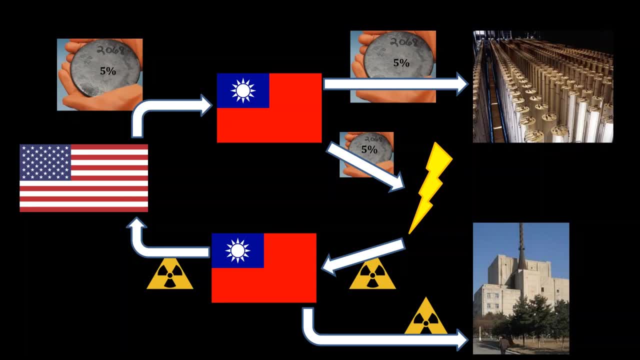 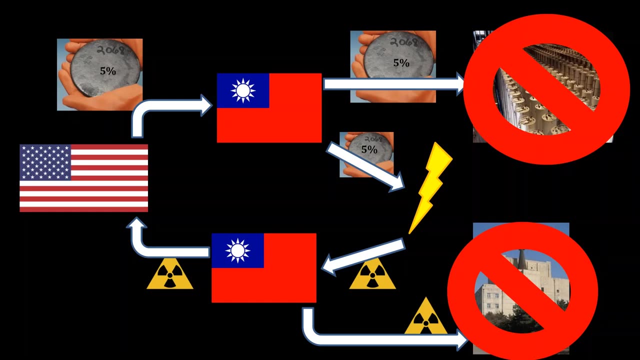 You need a plutonium reprocessing facility to actually take that plutonium that is inside of the nuclear waste and separate it from everything else Absent that, once again, you don't have a nuclear weapon. As a result, this system is proliferation proof.